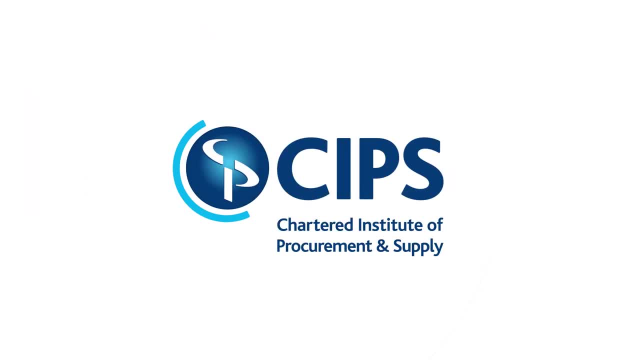 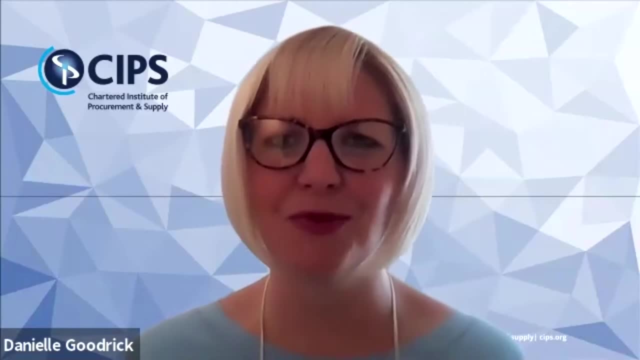 Welcome to the podcast today. I'm Danielle Goodrick, Knowledge Product Manager at Sips, and I'm joined today by George Booth. Hi George, Hi Danielle, How are you doing? Great? Great to have you here. To give you some background to George, he is the Chief. 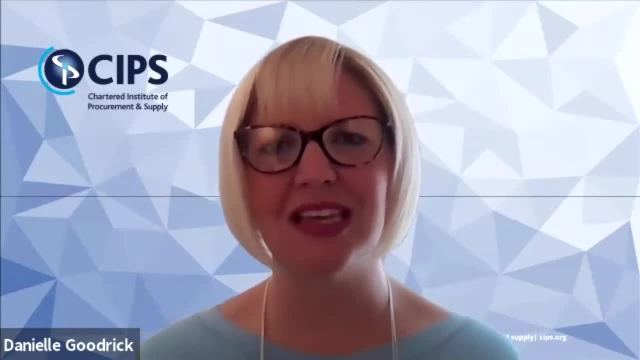 Procurement Officer for Lloyds Banking Group PLC, with 28 years business experience gained in global high-tech manufacturing and financial services industries, and specialises in procurement, sourcing, supply chain management, supplier relationship management, divestments and risk management. He leads a team of approximately 300 based across the UK and manages an annual spend of around 5.1 billion across more than 3,000 active suppliers. George features on the Sips Power List, and Lloyds Banking Group won the Best Practice in Procurement Supply Chain Integration at the Sips Excellence in Procurement Awards in 2020.. How did you find? 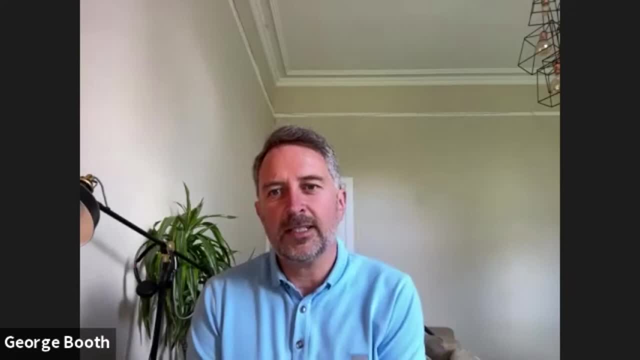 that process, George. As usual with Sips, it's a challenging process, isn't it, where we have to be very thoughtful on the team that we put forward. So the team write the brief, they present, I guess, the proposition into you guys for evaluation, and then they hold their fingers crossed. 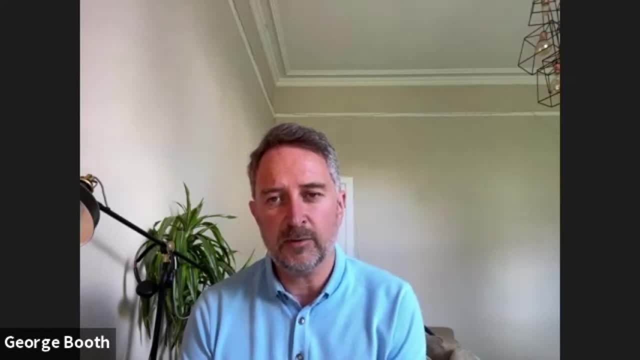 And we've participated with Sips now over many years in terms of awards. I've been a member for many years and a number of our colleagues go through it, So we're very familiar with the process. but there's a very high bar And you know we always submit four. 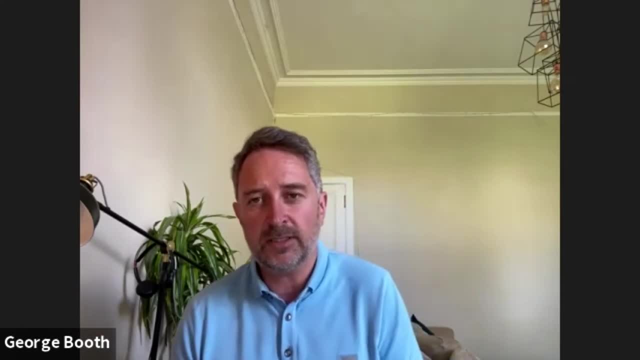 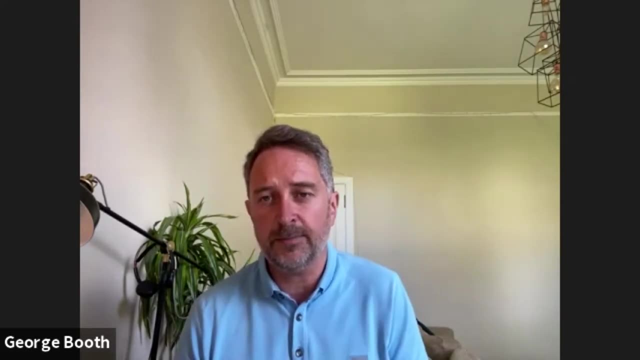 or five initiatives. It really motivates the team, focuses our minds And, of course, when we win an award we're delighted. It's a great level of kudos for the individuals concerned and the team. It helps with recruitment, It helps with retention And overall it's. 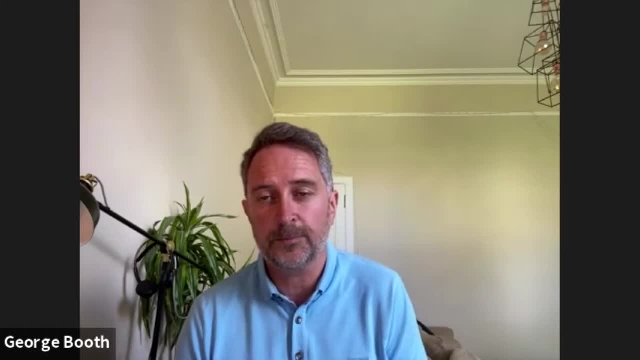 a great process. I thoroughly encourage anyone to go through. And can you tell us a bit about the award you won last year? Yeah, we won an award, for you know the innovation that we drove into. you know exposing risks deep within our supply chain. So everybody deals with third parties. We've got a lot. 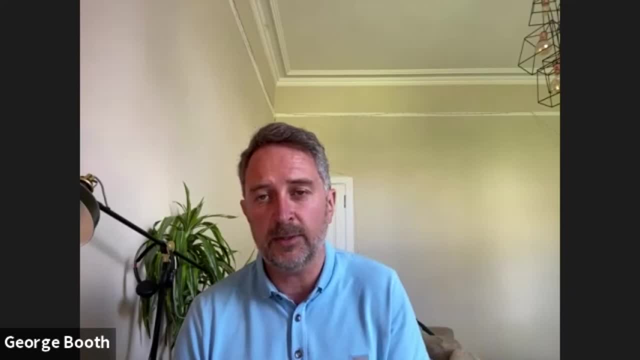 of third parties, but we were going beyond to try and determine, break effectively, an end to the process that we run, And we did a lot of collaborative work with our third parties to do it in a risk-based data-driven model And that's. 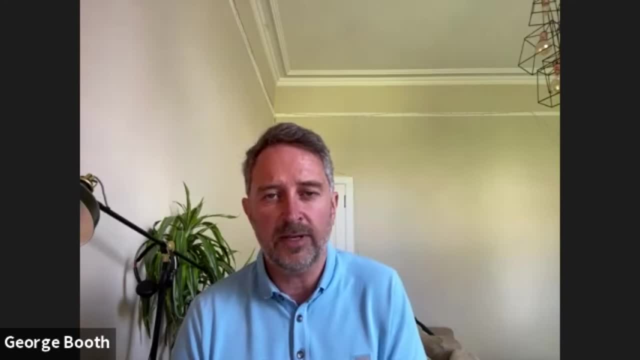 given us an ability to map out our supply chain in a granular level of detail that we've never had before, And it gives our businesses much more proactive insight to the risks they're going to have to deal with and the risks that supply chains represent. So I guess it's 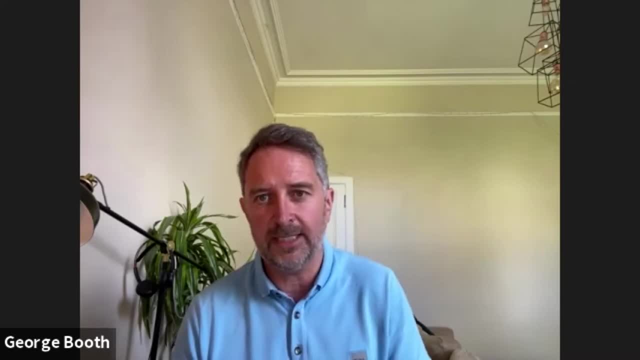 the first time that the judges had seen something like that, And we're now taking it to the next level of automating that and driving it at a larger scale. So, yeah, quite an exciting initiative And we also highly commend it, if you remember, for partnership in a game. 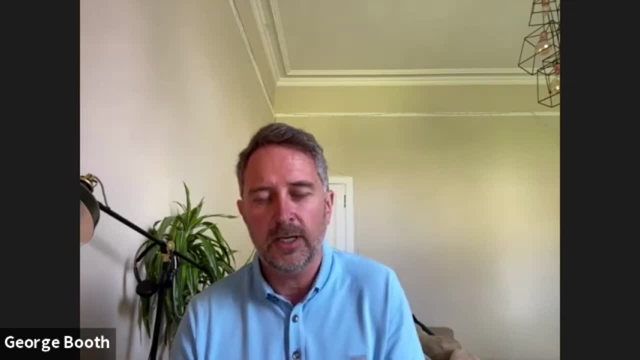 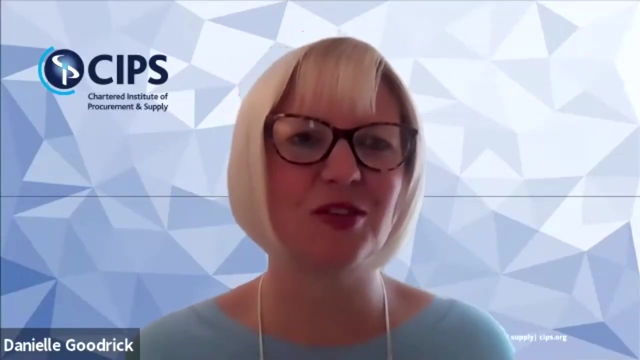 theory context, which is, I guess, today's topic of discussion. So, yeah, the team really love going to these ceremonies virtually, obviously this year compared to previous years, But, yeah, delighted with the win, Great, And the commendation really is what kind of leads us to today, So I'm really delighted. 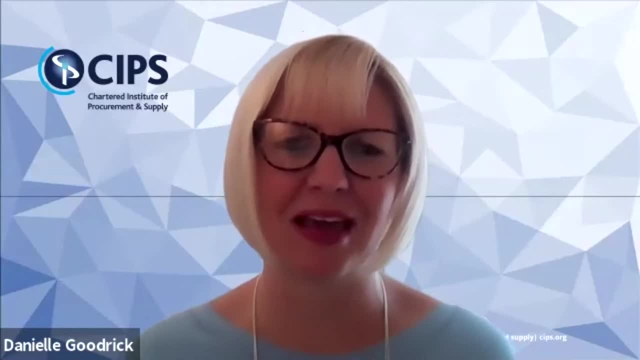 you've been able to join me to discuss game theories application at Lloyds Banking Group. George, TWS and CIPS have recently conducted their fourth annual survey designed to explore the awareness, understanding and application of game theory within procurement, And this year the results show that increasingly more procurement organisations are discovering 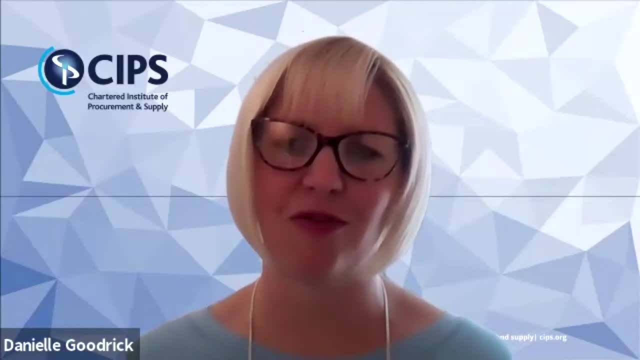 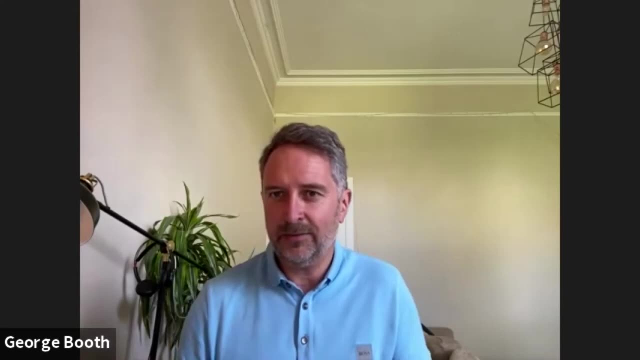 and applying game theory. So when did you come across game theory for the first time? Well, the first time was probably in school. I remember the Prisoner's Dilemma. It's a very famous form of game theory, And I studied economics at university along with marketing. 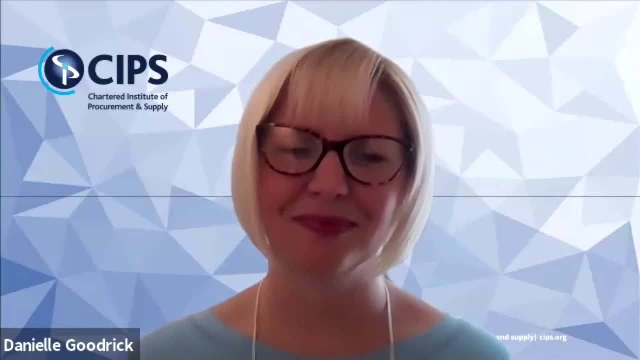 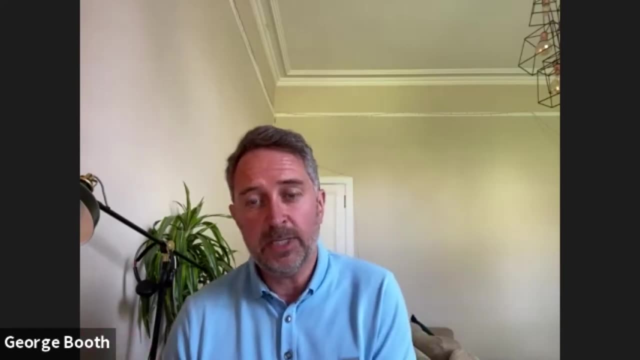 So it was a big part of the course And I kind of hadn't really appreciated, probably until seven, eight years ago when I was at a future CPO event, I met a peer working at a large UK automotive organisation who had actually implemented a game theory modelling. 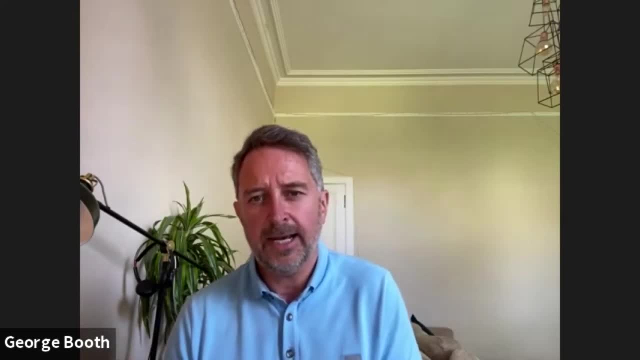 tool and methodology. So I started looking into it a little bit more and quickly realised I've been applying game theory in my social career without realising it. Most buyers out there do it And game theory is really simple at one level where there are rules of a game. 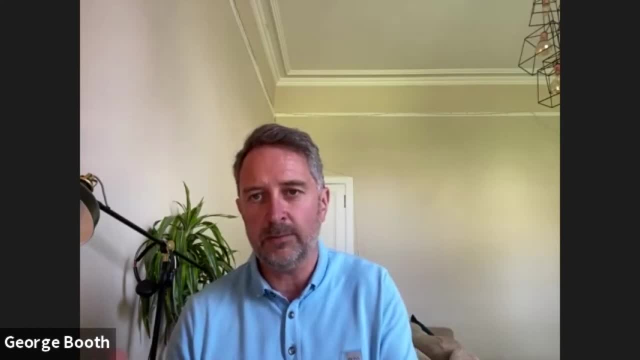 or an interaction typically between a business and the supply market, And we could see the effect and the impact it could have to drive more positive outcomes for, ultimately, our customers or business clients, And it was a much more collaborative way of looking at achieving better outcomes. So I started looking into it a little bit more and quickly realised 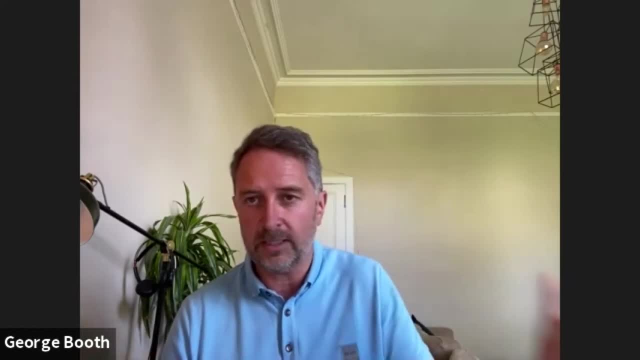 it was a much more collaborative way of looking at achieving better outcomes, where you've either got, on the one hand, monopolistic situations or a very diverse, rich choice in a market and everything in between. So yeah, I guess I've been familiar with it for 20, 30 odd. 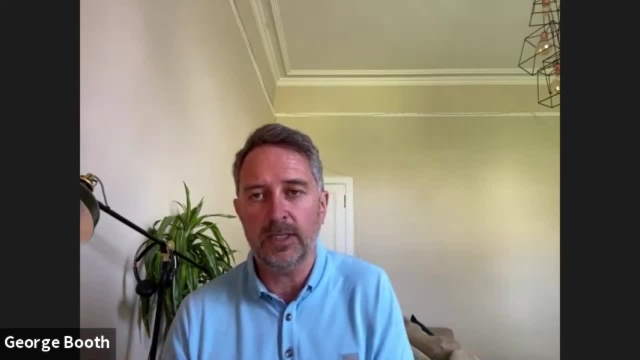 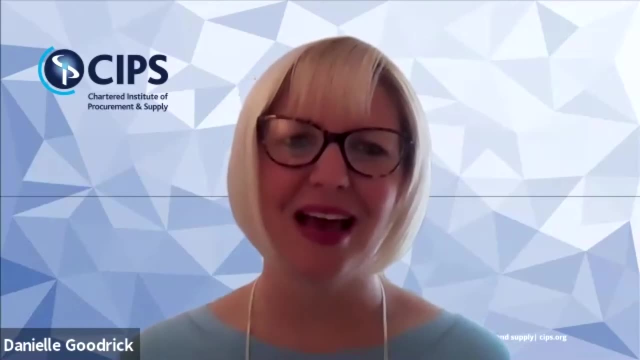 years, But in practice, profession, I've been implementing it with the team here at Lloyds for probably the last six or seven. That means you've been at the forefront of the development And our report highlights this year that more than 80% of game theory users started applying game theory over the last six years and more than 50% started in the last 30 years. So why did Lloyds Banking Group look into it back then? I guess we're always looking for the edge or the next thing in procurement. And again, 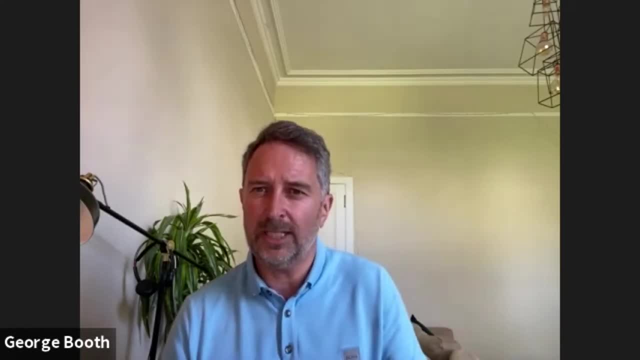 like I said, we were doing game theory without articulating it or really understanding how it worked, And it's only when we sat with professionals who were, you know, PhD qualified mathematicians, statisticians, game theorists that are, you know, qualifications in it. now, 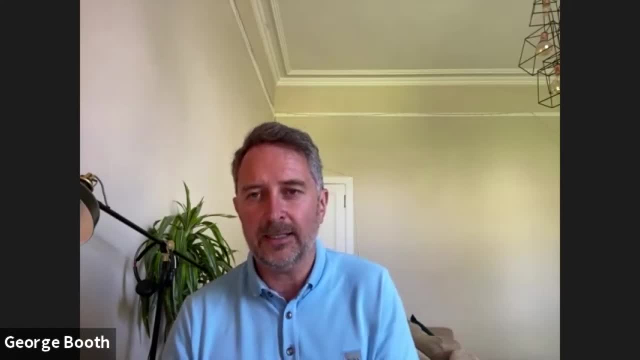 that you can achieve. When we realized that it was an opportunity to upscale our team And I've got a community of about 150 buyers, most of whom we've now trained through formal game theory methodology and practice, the vast majority of whom have undertaken sourcing. 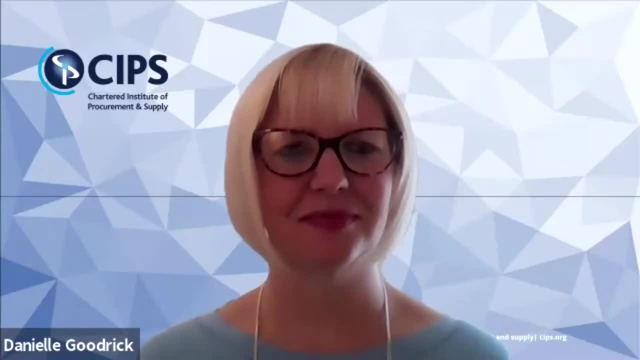 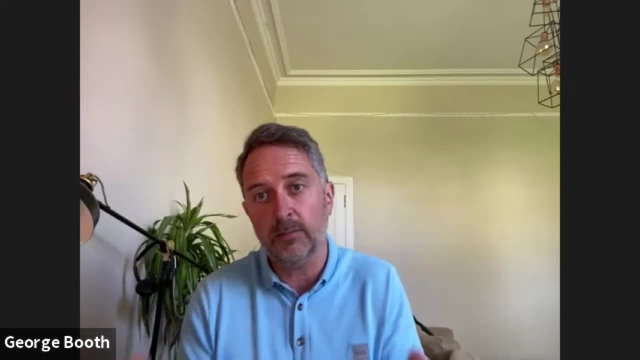 exercises applying the core principles of it. So we saw it as a way of ultimately driving better outcomes for our business, our customers and our suppliers, Because the more you have an open, transparent set of rules governing the ultimate aim for win-win outcomes, the better chance. you're going to have a positive reputation in the supply markets, where you can attract the very best talent to work for you. you can attract the best suppliers to provide services and goods to you and you can get the best collaboration with your business. 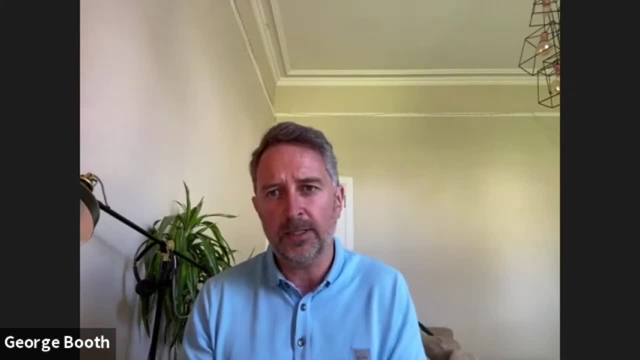 clients, Because often in sourcing or procurement the rules aren't very clear And it's not obvious why a company won over another. Yeah, Yeah, Yeah, Yeah, Yeah Yeah. Or you didn't pre-position the rules up front and there are disputed outcomes at the end. 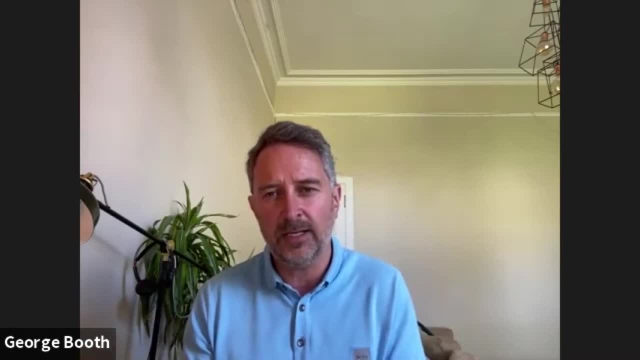 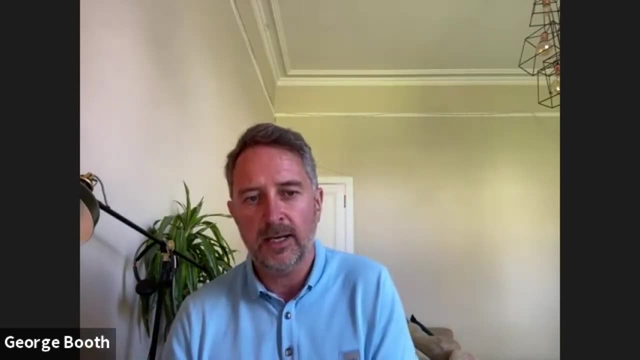 And quite often the process can end in a bit of a negative way, But ultimately we've got a long-term view in mind that we want to be professionally represented in the supply markets. You know, during my tenure in this role and for my successor and beyond, it's 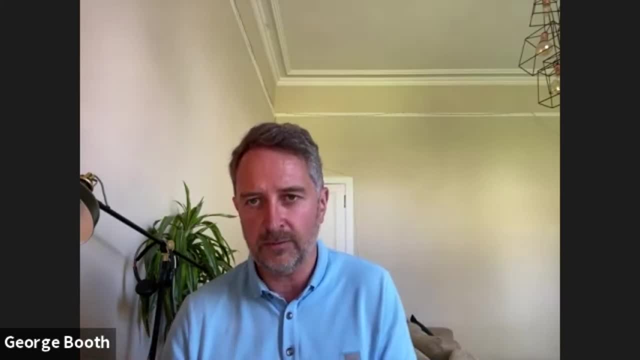 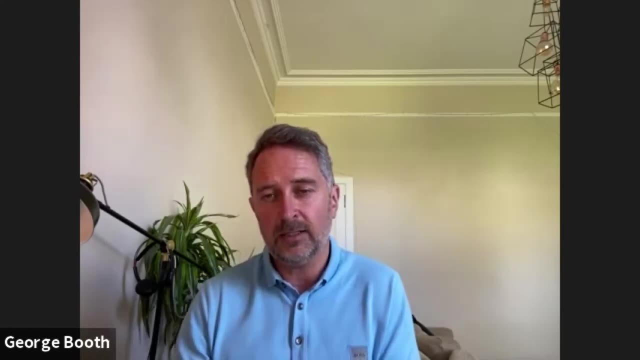 really important that Lloyd's reputation remains very positive And we saw game theory as a part of the way we have to drive them to the next level of competence And it attracts, like I said, people to come and work for us to learn these skills. 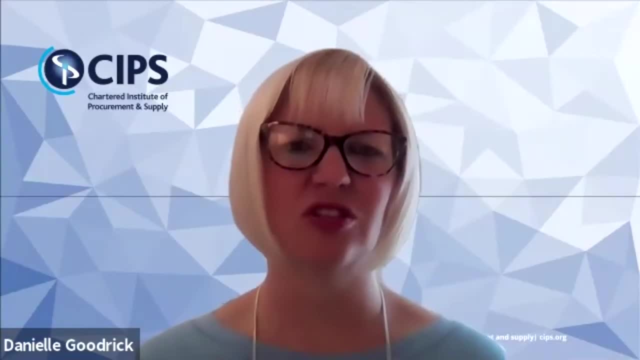 Most definitely, And although most professionals have heard of game theory before- and we've spoken about this to our professionals for some time now- only 50% actually use it in their day-to-day job, according to this year's results. But you've used it for some time, So what does game theory really mean for you? 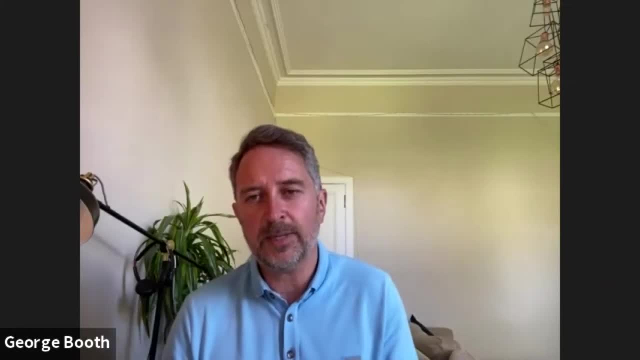 I'd challenge your results right, Because I suspect 100% of the time you've used it for some time. So what does game theory really mean for you? I'd challenge your results right, Because I suspect 100% of the time you've used it for some time. So what does game theory really mean for you? 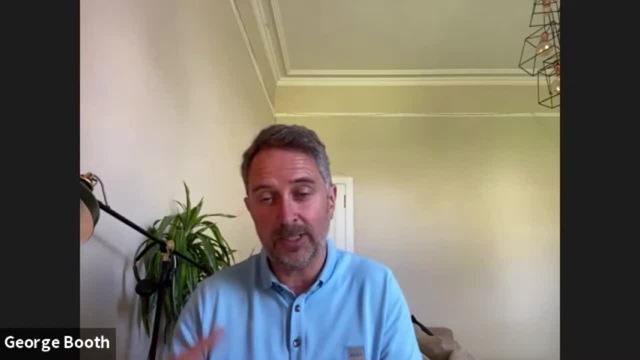 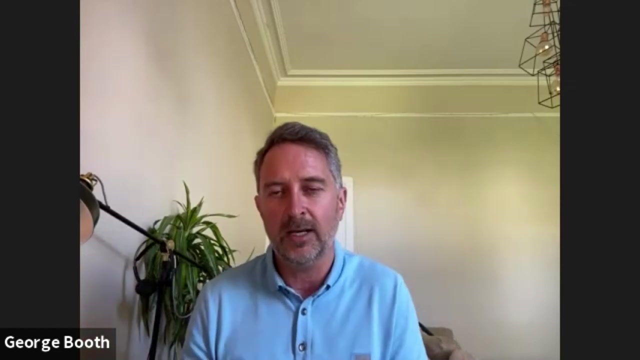 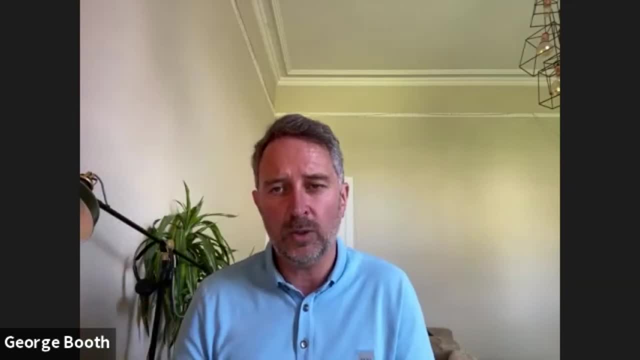 Then there was that deux of b ride: efficence, the bad productions and the best productions. There was the opportunity for the two of us, And you know so that two of us, the two of us, the two of us, the two answer the question: how many companies? how many companies? that doesn't take, although there are activities they really need, out of我觉得, yet of. 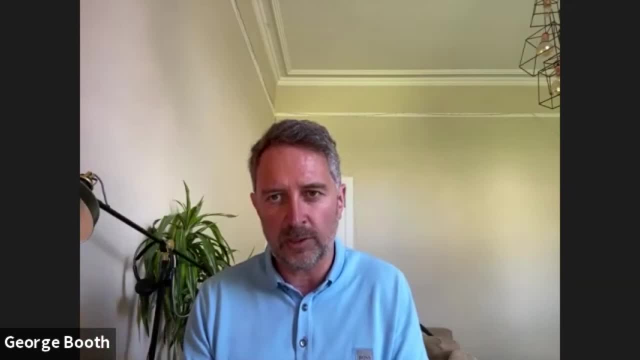 the design of these on the customer so that they can serve their employees by combining the needs. the design of these on the customer so that they can serve their employees by combining the needs possible, and communication of that requirement is really key. it's not all about getting the best. 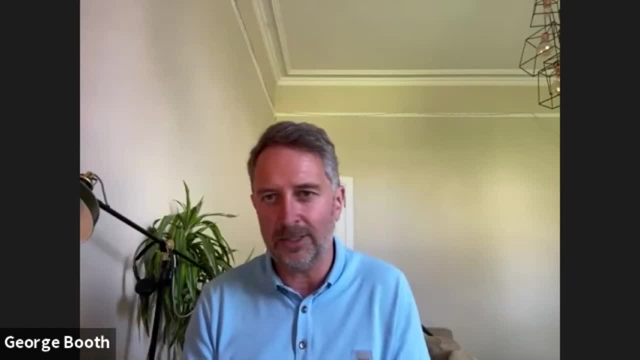 price, the best quality, the best service, the best innovation, access to the best people. it's a balance across these factors and you have to ensure that you know your scale and your presence and, most importantly, reputation in the market is as high as possible, because your reputation is what follows you as an individual, what follows you as an organization. so the 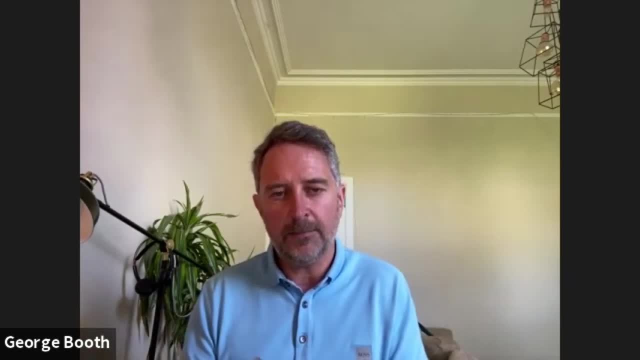 suppliers, once they understood that that we've been really genuine, have bought into it. suppliers have been through many game theory based sourcing exercises multi-times over and i've had loads of conversations with you know senior people in our supply partnership taking game theory to heart and actually tried to implement it- and in some cases very successfully- into their businesses. 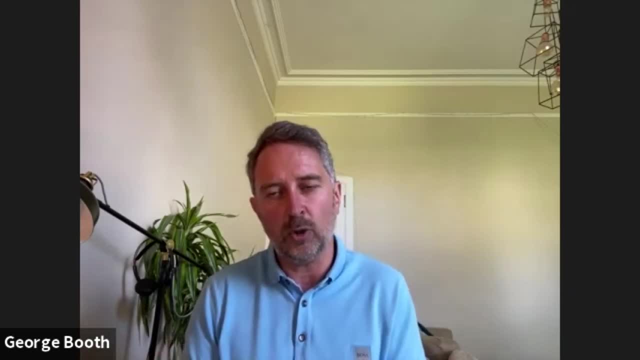 so it is a methodology. like i said at the beginning, it's always been there that people haven't quite realized was couched in the principles of game theory. but when they've actually looked at these principles and then professionally trained and adopted them, it's, it's become very obvious that, ah, why weren't we doing this, you know, in the past? 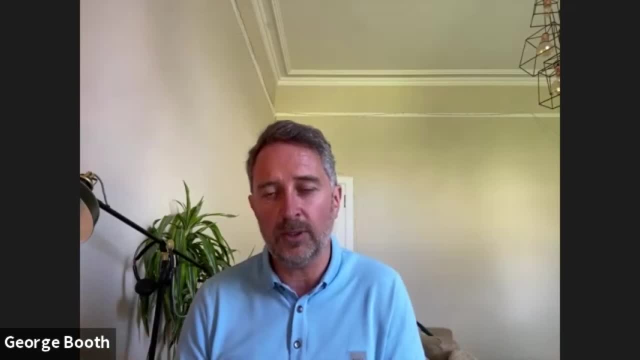 so the suppliers will come on board, they will work with you and because more and more organizations are doing it, by extension, they've experienced it. so the ecosystem globally around us is really growing and you're going to be in the minority if you're not taking a more applied game, theoretical, 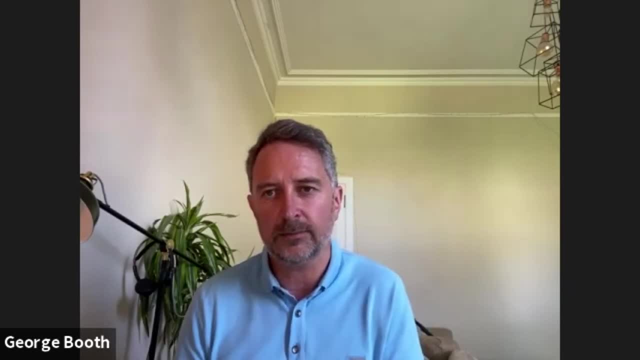 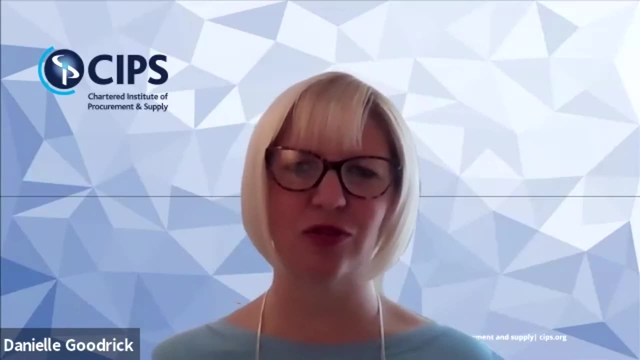 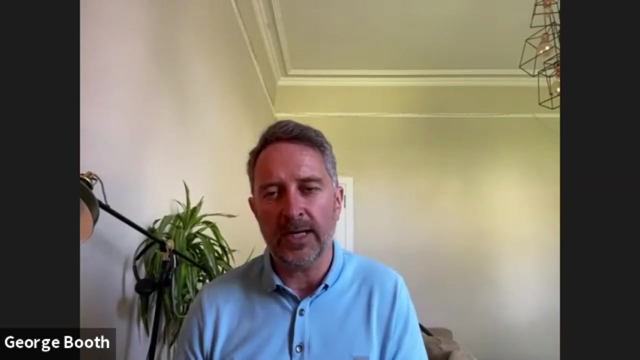 approach to your sourcing procurement exercises, And you seem to have really pioneered this um approach. so how have you organized the upskilling of your teams and incorporated game theory into your team's training? I was fortunate that I got sponsorship from my, my CPO at the time- uh, chap called Michael Whitby. he 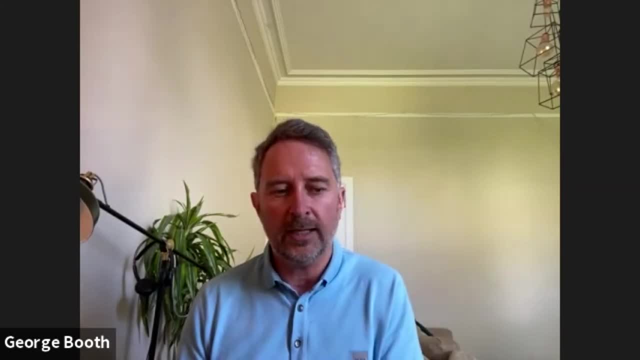 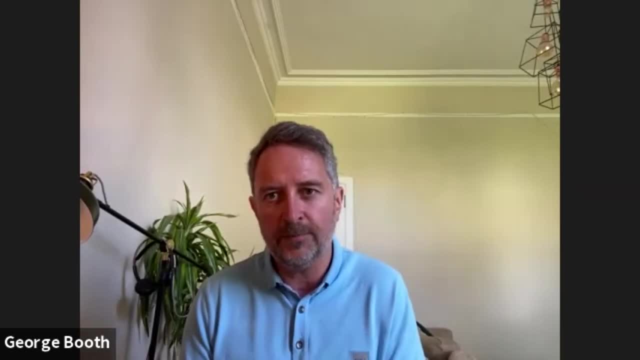 the merits and he quickly understood the merits, and he quickly understood the merits and he quickly gave me the sponsorship to go away. we pulled together a small team, um of enthusiastic peers. we then, you know, asked for volunteers from our buying community, um, and a number of them, you know. 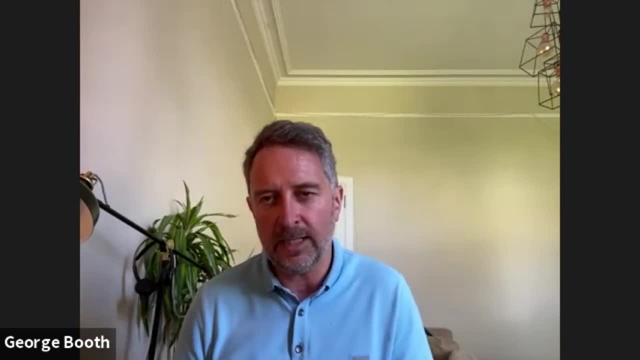 really got enthused by it. we then partnered with our game theory provider. we established a bespoke training course, a qualification that you can get um, and we've now got experts who have become training the trainers. so we now train our own people, um, in the method, and it's something you have to have as part of your culture, part of your DNA. 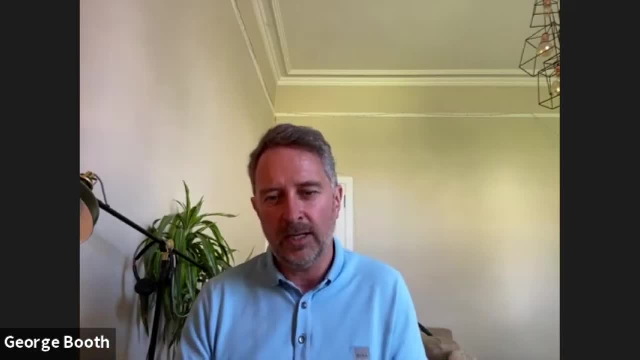 it's not a course you go on and hope to remember. it's how we do business and it's applicable to the very smallest of spends and most simplest of tasks, right through to the most complex thing that you will buy. so I think, just having a kind of enthusiasm, a level of sponsorship over it, Danielle. 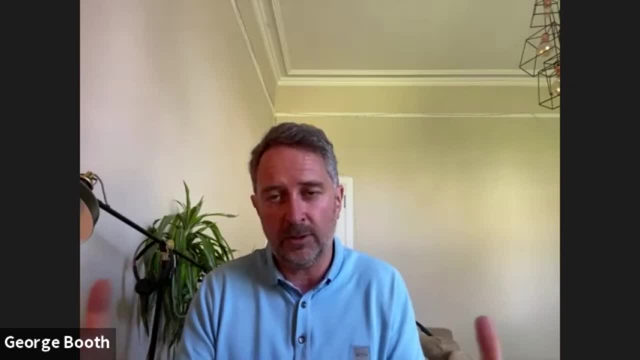 is really key, uh, right from the executive running the procurement sourcing function right down to the most junior buyers and the most senior buyers and the most senior buyers and the most senior buyers and the business execs that sponsor us and ultimately pay the bills um, they all have to buy. 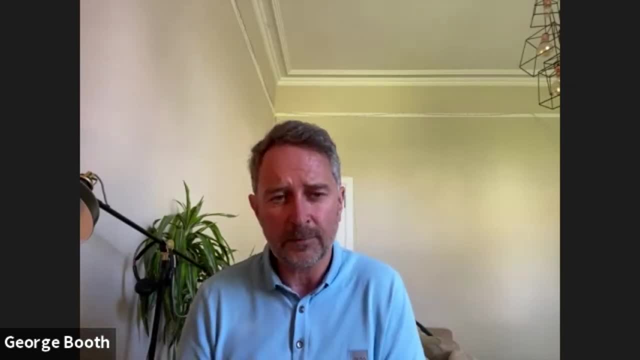 into it. so it's a cultural change. it takes time, you'll have some bumps in the way, but if you stay, you know a believer, if you demonstrate good results, like everything, it'll eventually be embedded as part of how we do things around here. and from what you've talked about there, you've 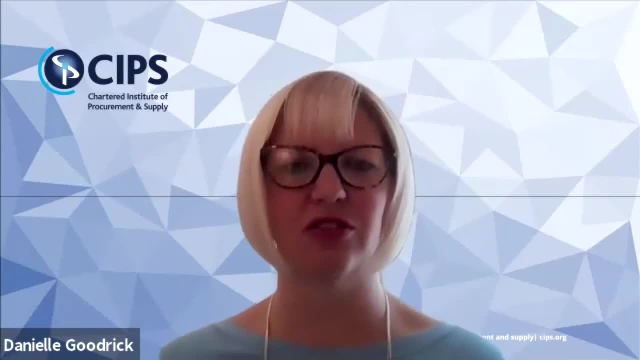 built up a significant in-house expertise where you've got trainers who train your team. it's been part of your DNA, but it'd be interesting if you could tell us in which categories, or perhaps market situations, you want your teams to adopt this approach. is it internally and externally, or is it just more? 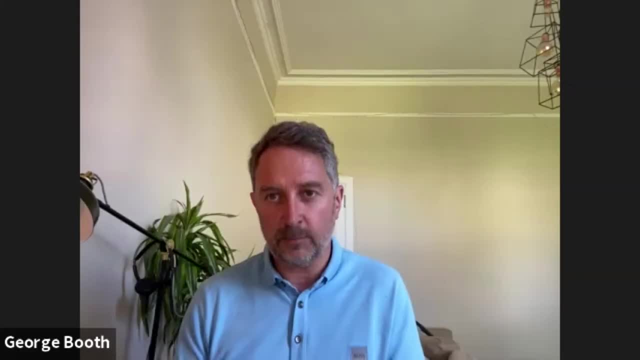 supply market. it's, it's supply market for us in the main. um, again, the very core principles, often to make sure that we fairly, ethically, sustainably, transparently source in the markets. and you know the the sense of achievement after an exercise is shared often by the suppliers and the procurement professionals, along with our business. 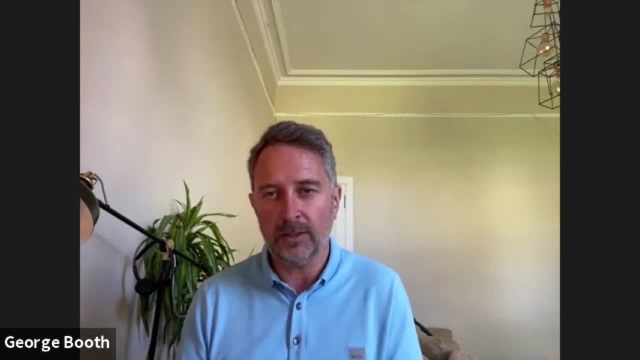 clients internally. everybody will sit down and go wow, you know, that was an amazing experience. i've learned what a kind of dutch auction is, or an english auction as part of game theory, and how we drive competitive pricing um and and sometimes the the path to get the best outcome is not very 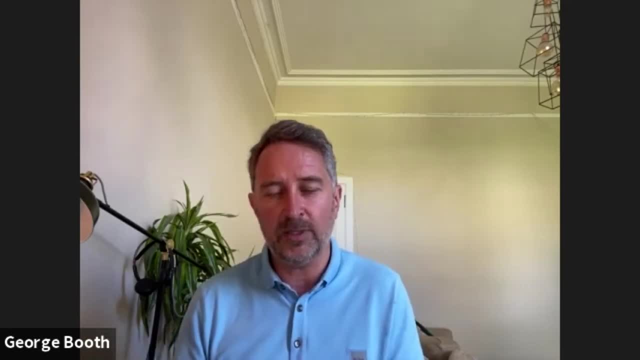 obvious. so i think it's that shared sense of achievement and learning and sustainability as you take it on to the next exercise, and i think it's a very important part of the exercise, and i think it's a very important part of the exercise and i think it's a very important part of the exercise. 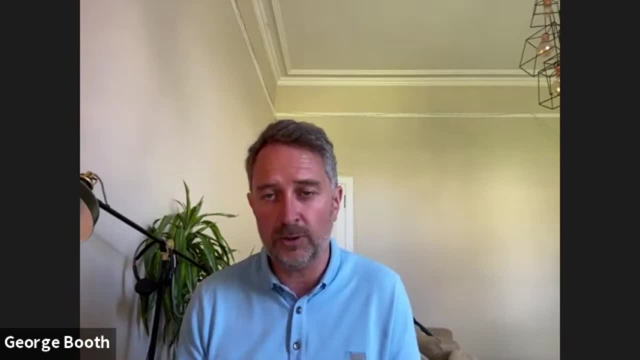 so everyone in my organization, uh, it's open to them. we do it across all categories, we do it in all markets. um, and i'd venture to say now pretty much every supplier that we deal with has gone through an element of a game: theoretical based sourcing interaction. um, walked away learning a. 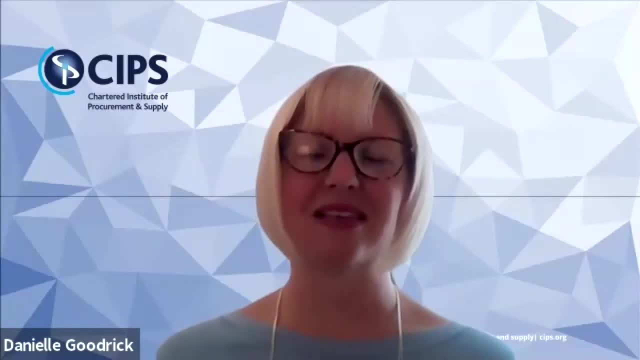 bit more about it and that that's intensified over time. i'm assuming that to reach that point, um, if we just talk a little bit more about that- and i think it's it's a very important part of the experience- and talk a little bit more about that and i think it's a very important part of the 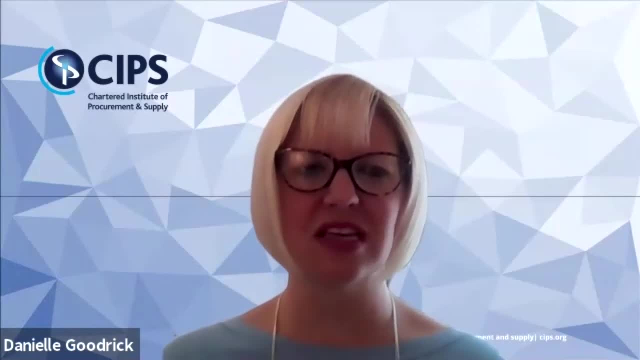 experience and talk back on the report and the findings this year then, before we close. so more than 60 percent of respondents believe that the use of game theory in their organization will rise in the future, either because they'll either introduce it or intensify it. so just to close them, what would be your recommendations to them and how should they? 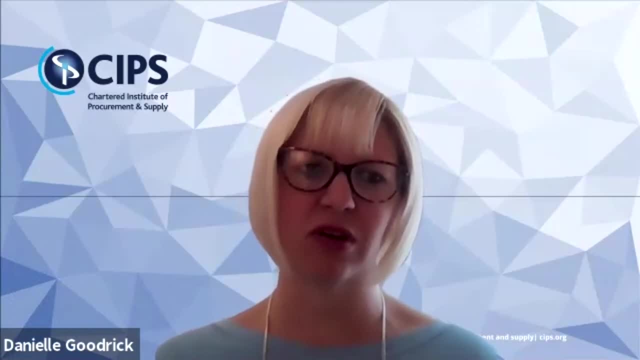 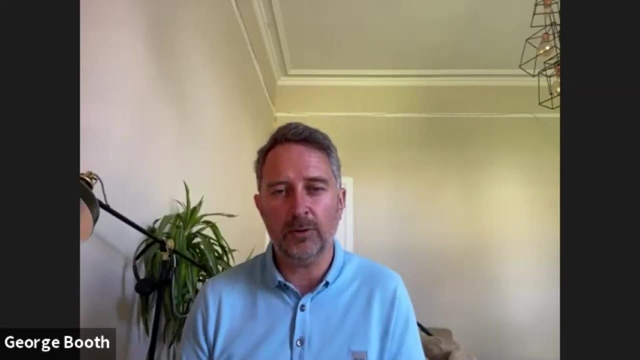 get started or how should they roll it out further in their organizations? the first thing i would say is go and speak to the experts, um, go to speak to the people who run the practices out there, and, And they're easy to find. There are many we've partnered with. you know one in particular. 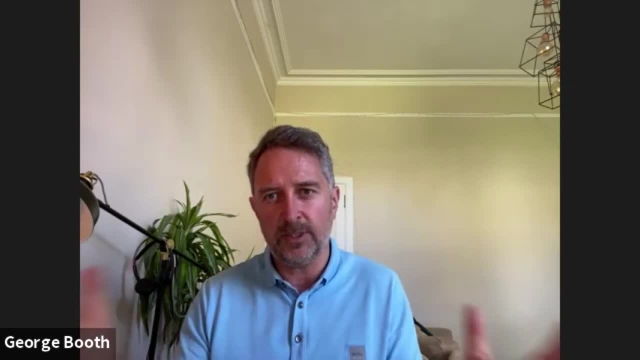 The second thing, then, is translate that for your leadership team, So as a community, within your CPO line, see where there are voices of challenge, voices of support, But as a community, you know, immerse yourself in it, Go on a course, learn about it, run an exercise. 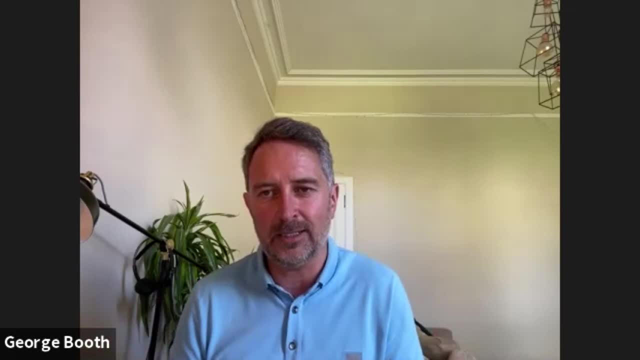 And they have game theory games that you can play without necessarily going to the market. And if it's for you, if it fits your culture, if you think it can enhance the outcomes you achieve, you then have to talk to the businesses that you work with, because they're a key part of it. 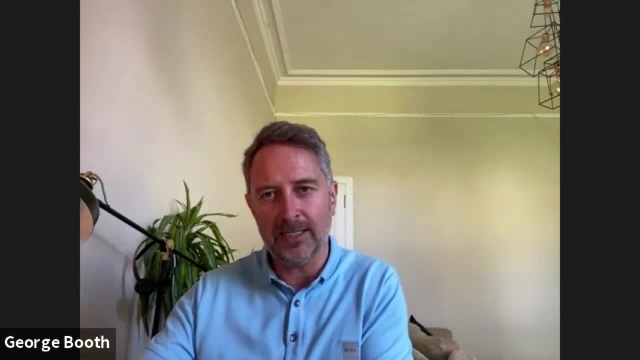 as well as obviously then the suppliers, and explain it. The worst thing you can do is keep it as a secret in some black box and think magically you're going to get amazing outcomes by applying the theory just in the procurement sourcing team. You have to bring your business. And the suppliers with you. So the second key question is transparency. You know, be open, be honest about it and then just rigorously reinforce it, sponsor it, highlight the colleagues who have really stepped up. You always get early adopters, Danielle, I guess. 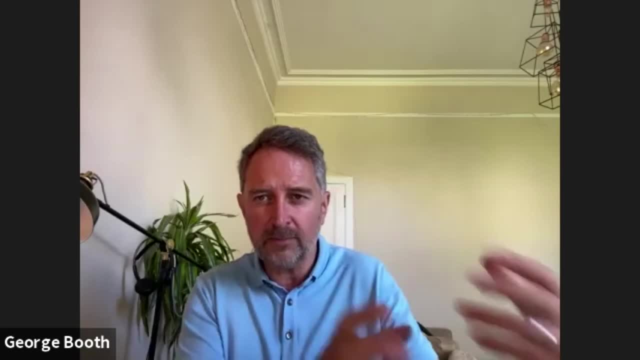 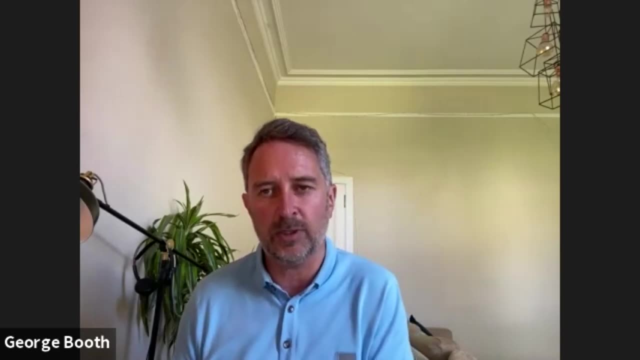 And you know, encourage them, nurture them, give them the kind of space to explain what they've done and what they've learned, And probably the last thing is get a sustainable educational investment program in it. You know, put some money behind it. 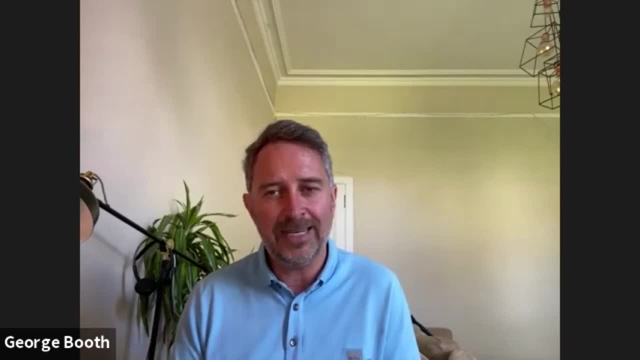 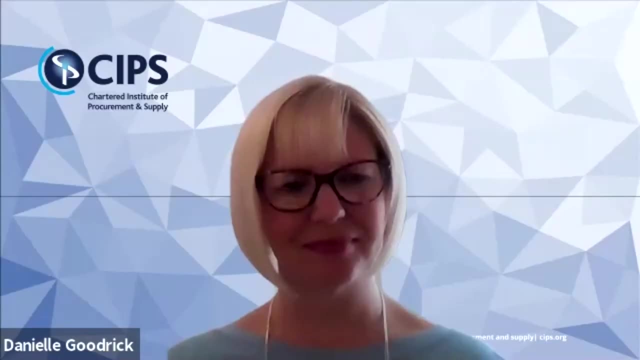 And it's all part of it. Yeah, It's all part of development and growth and retention And what is a very tight talent market, Largely the UK. for us, we want to attract the very best And if people do leave us, we want to export a really good story as to the skills they've learned, the talent that they bring elsewhere.